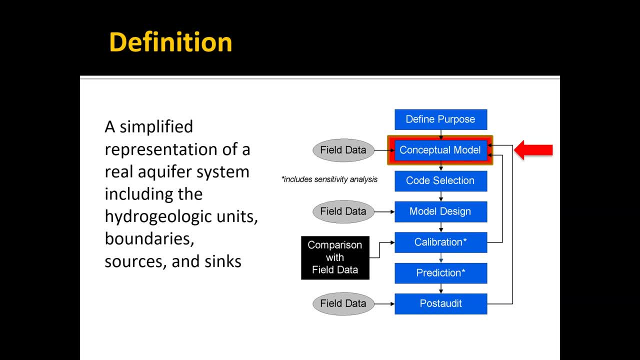 and to come up with, as the note says, a simplified representation of your aquifer system, And you need to identify the hydrogeologic units, your boundary conditions, sources and sinks and basically identify what are the most important parts of the modeling process. What are the most? 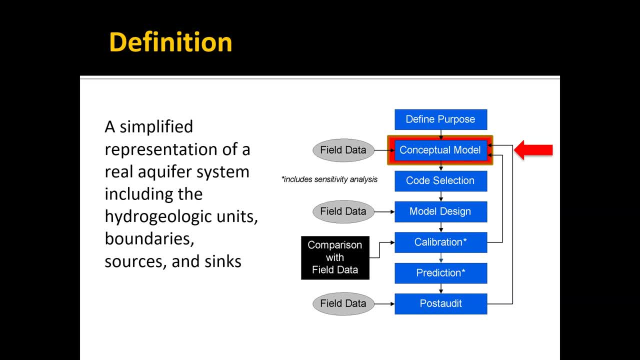 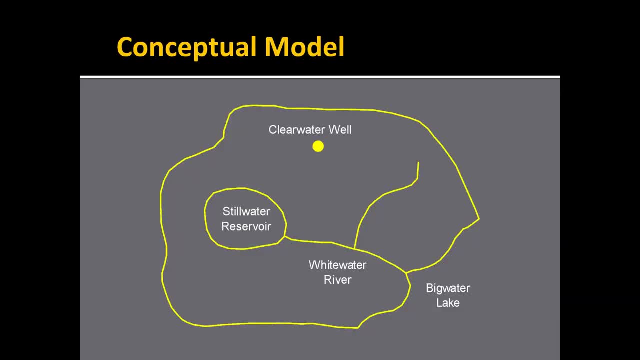 important features that need to be included in this model, And there's a lot of really important judgment that goes on as part of this process. So this is kind of one way to think of a conceptual model. It's kind of like imagine yourself with a groundwater modeling team and you're sitting in. 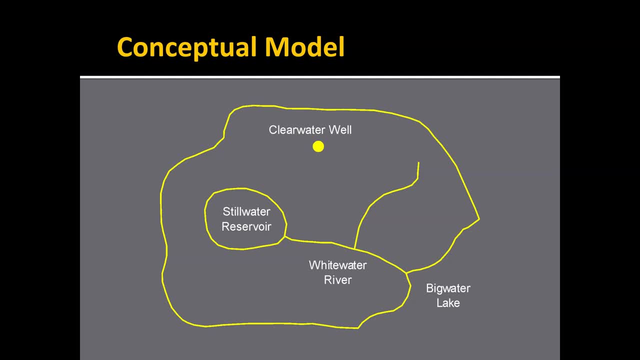 a conference room and you get out a marker and a whiteboard and you you sketch out: okay, what are the critical features here that we need to include in this model? It's more complex than that, But that's that's kind of how you start. You identify your boundary first of all, And that 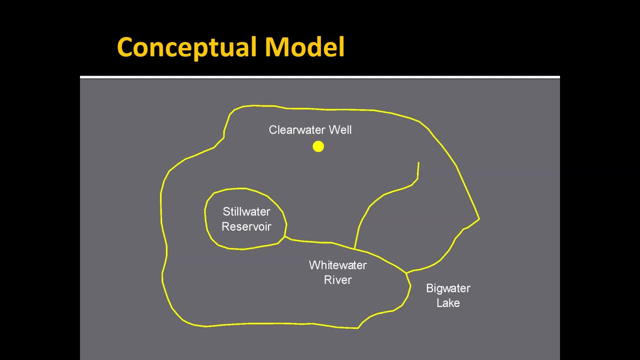 is. that's such an important thing that we are going to spend a lot of time talking about that over the course of the semester. And you know what are the primary rivers and streams that you're going to use for your modeling. And then the other one is: what are the major reservoirs and streams that you're going to use to mini. 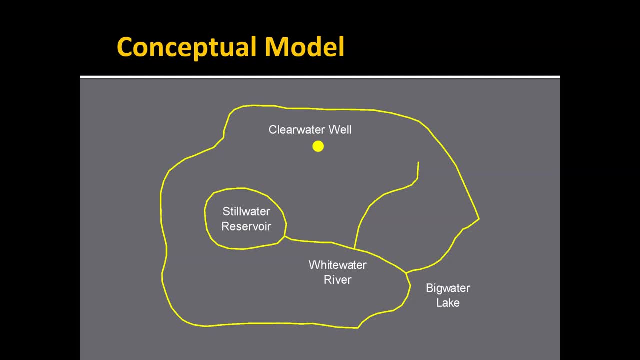 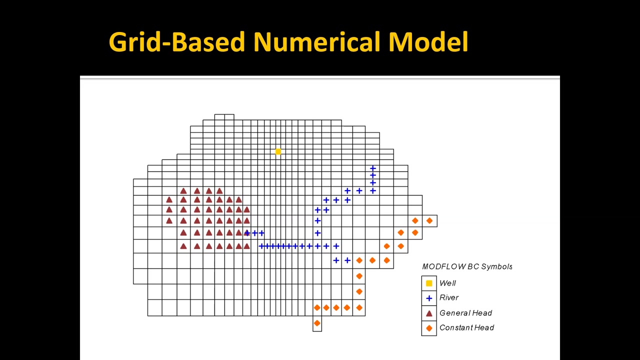 to feature water bodies that interact with the aquifer, what about the stratigraphy wells? of course, all this, anything, what are the main things that impact our model? and then, once you have that established, you can then convert that into a grid-based numerical model, as shown here. so this, we're actually going to build a model very similar to this. 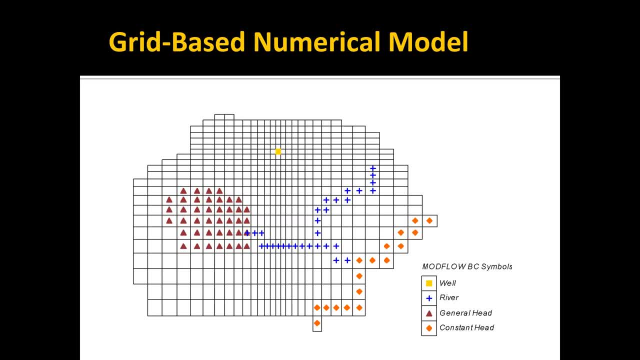 as one of our exercises in the class. but as you'll see in this numerical model, if you look at those symbols that represent different, different features of the model, you know those are first represented in your conceptual model. so just to give you a little better feel for this, let's look at a few sample conceptual models. 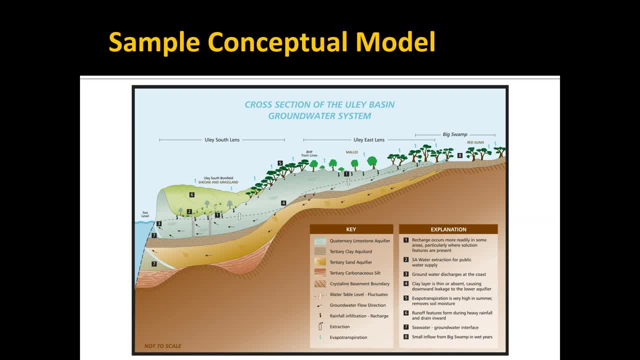 um, so here's one. i believe this is in south africa. i found on the internet. it's a cross-section through a real site and someone has gone in and the real system obviously is much more complicated than this- but identified what are the principal hydrogeologic layers. 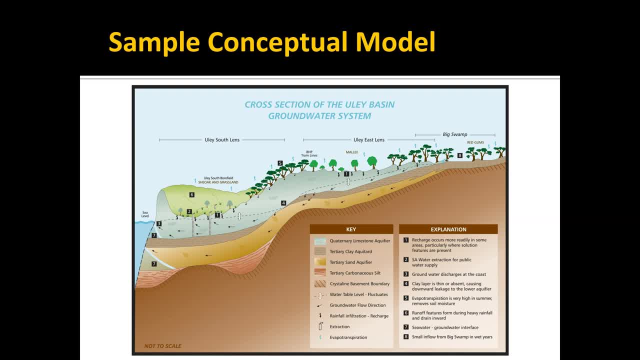 or features in the model where the water comes from, how it enters and exits the system. in this case, we have recharge and evapotranspiration through the trees, there's some pumping, that goes on, and then there's actually, in this case, interaction, uh, with the ocean, and you'll notice. 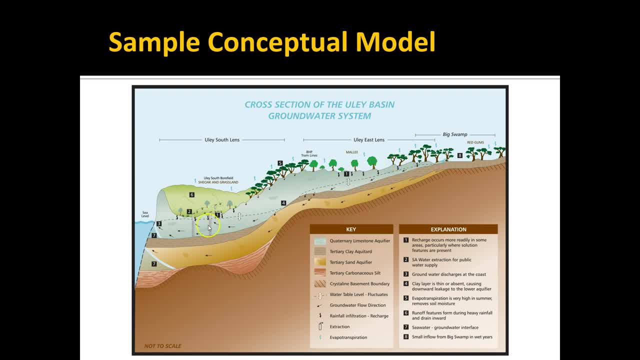 there, there's a, a low, an upper aquifer, a sufficient aquifer that's unconfined, and then the lower aquifer is exposed to the upper aquifer. and then there's these: there's a confining unit and then a lower aquifer that, in, at this location here, is exposed to the upper aquifer, but other 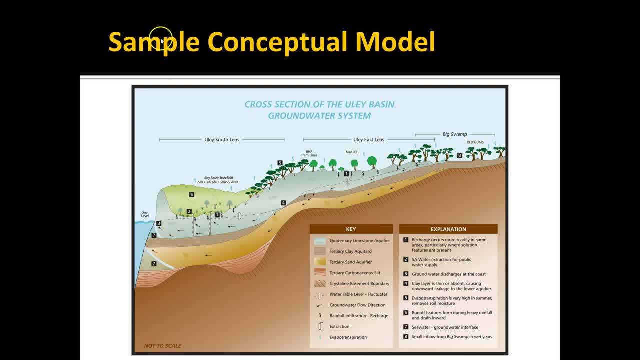 than that, it's confined and then it's assumed that you have two separate uh salt water, fresh water interfaces over here. so somebody has gone to some lengths this to sketch this out and analyze the underlying data to come up with this, and then we can uh take a little time to show you a little bit of the whole picture. 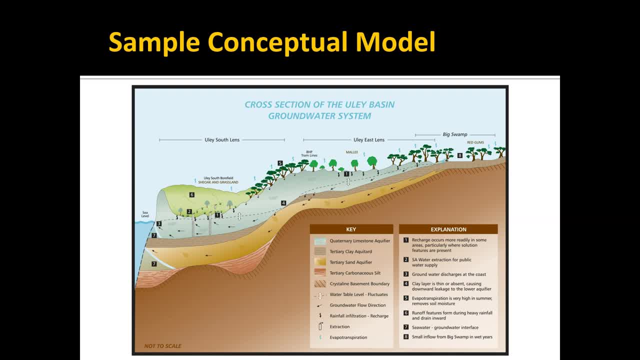 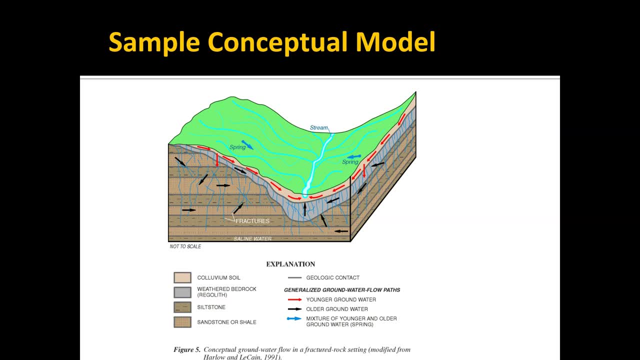 and then, uh, how the water can come up and out, and i hope that you can see my work here. next slide: um, the water can come up and out of the water and can then go, uh, into the water. so you can see how it's separated here and you can also see the different ways that it can be. 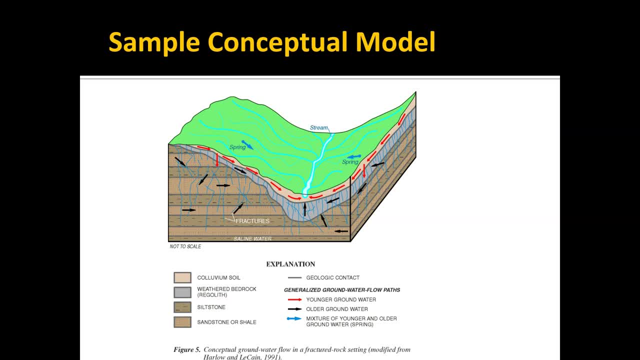 separated, and you can see how it's separated on the ground here, but the only thing is that it's not lose, because the water is just a little bit wet right now, so you can see that that's what's layer. there are springs and streams that interact with this system, and this is a 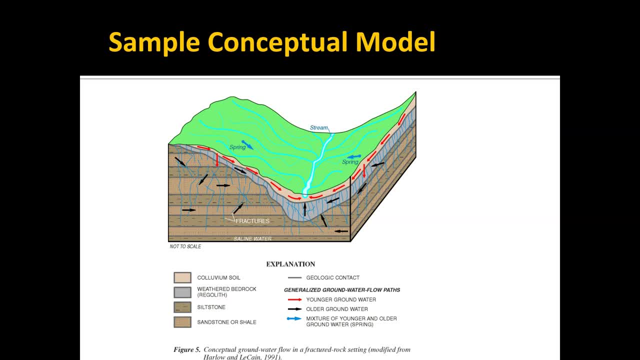 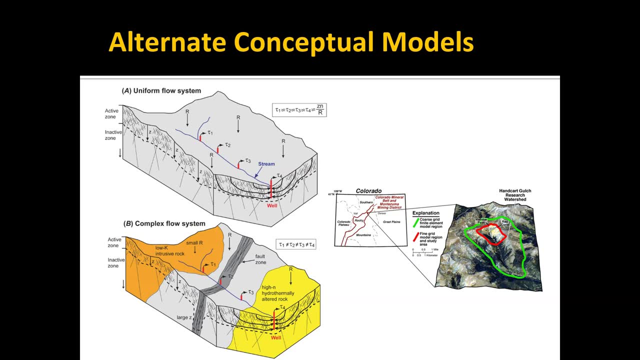 conceptual model was developed by someone back in 1991 and this is one I really like. sometimes it pays to have to look at alternate conceptual models, and typically this means we have like a simplified representation and a more complex representation, and so part a is more of a simplified representation. 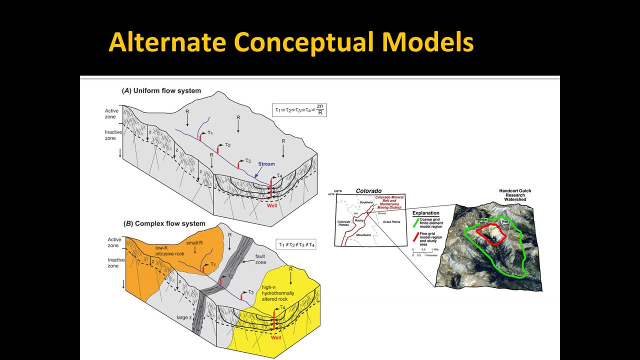 there's a stream that where the, as you can see, there's recharge entering the system and then it is exiting the system by discharging to a stream in the middle of this basin, and you know, altogether it's, it's a pretty, there's, there's, there's also an 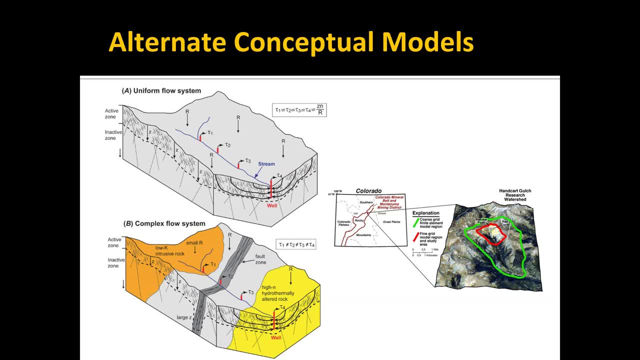 upper and lower zone. lower zone is an inactive zone. there's not a lot of flow occurring in the lower zone. most of the groundwater flows through the upper active zone and that's a. that's a real simple way to represent the system and then in in part be you'll notice that that they've added some more. 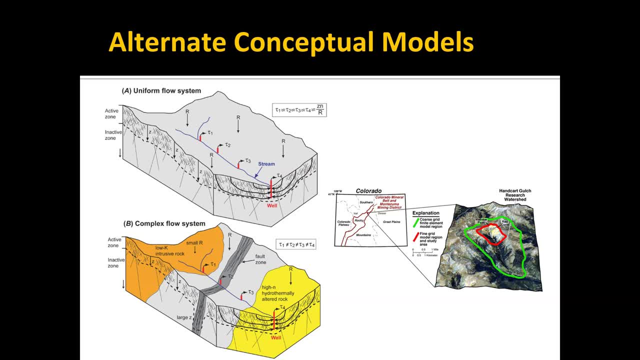 detail. there's a fault in the middle, and the different colors represent zones with with different hydraulic conductivities, and that adds a little bit more complexity to the conceptual model. now why wouldn't you always just use the more complex model? well, no matter what you do, there's some point in. 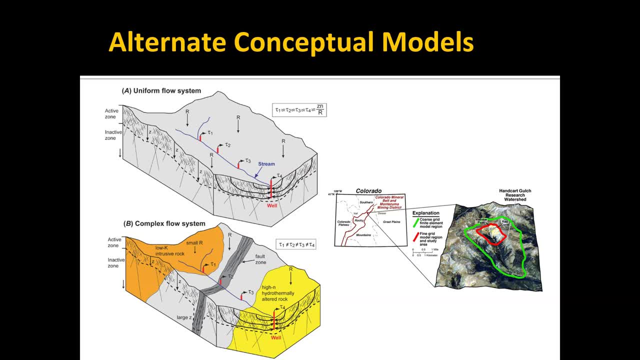 the process where you have to make simplifying assumptions. it's just a matter of where you draw that line, and determining how much detail you put into it really depends on the objectives of the model. you know what is it you're going to use the model for. the more complicated you make the model, the more 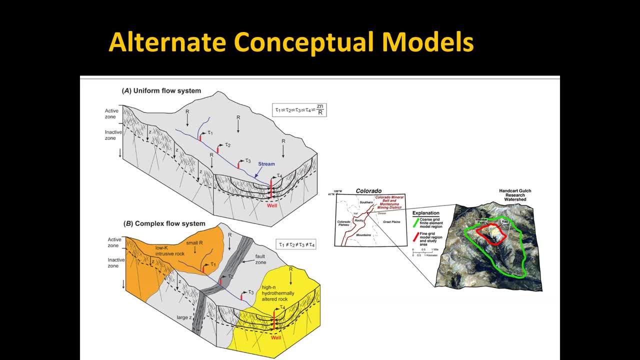 expensive and time-consuming it is. and for example, for this lower model that has the multiple zones, do you have a means of estimating the hydraulic conductivity in the different zones and you have a water level measurements in observation wells in each of these zones that you can calibrate to to kind of differentiate the flow in the different? 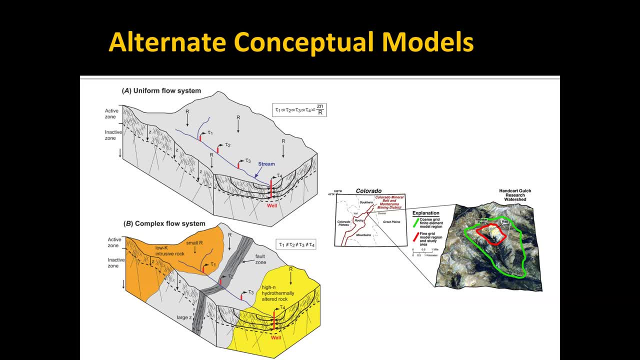 zones and, you know, maybe, maybe you don't have enough information to to really characterize that, and so you stick with a simpler model. or, in other cases, it's modeling strategy: to start with a simple system and then just gradually add complexity as you go along. that's, that's a technique that I quite like to use, and 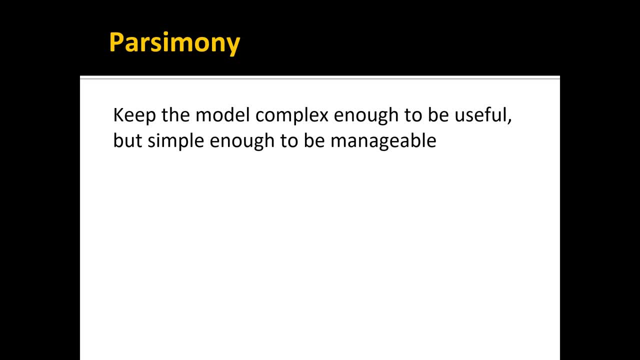 as you build your conceptual model, there's this concept of parsimony. parsimony, however you print different people pronounce it differently, but the idea is finding a balance beat between simplicity and complexity. you want to keep the model complex enough to be useful, but simple enough to be manageable. 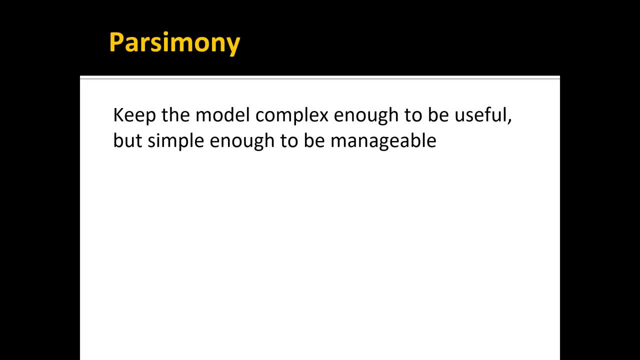 and how do you? what's the best way to do that? well, that takes experience and judgment. if you don't, if you make your model too simple, it's not going to be able to provide you with much useful information as a, as a tool to simulate what it is you're trying to do with your predictive model, for example. but if you 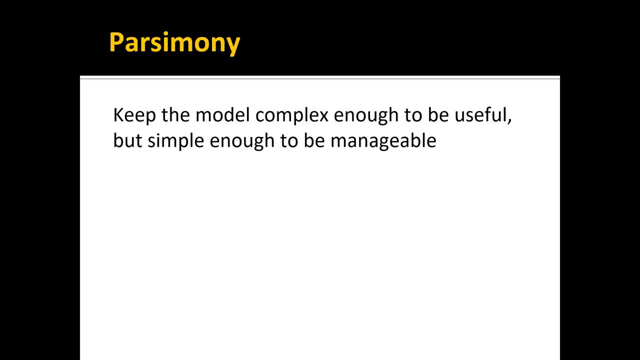 make it too complicated, then you can really get bogged down. it can be stupid, slow to run, it can be expensive and time-consuming to set up, and so there's there's a balance. you have to pull together there, and when I think of this, I'm often reminded of a famous quote by Albert Einstein: everything should be. 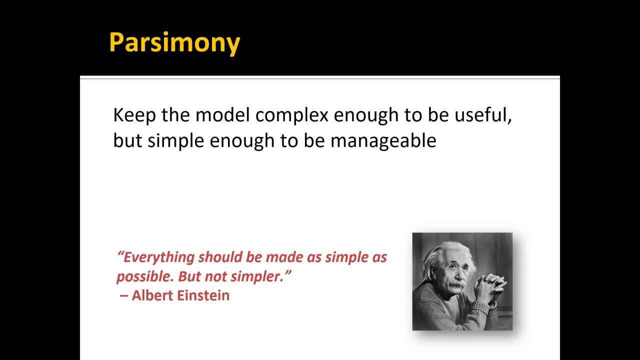 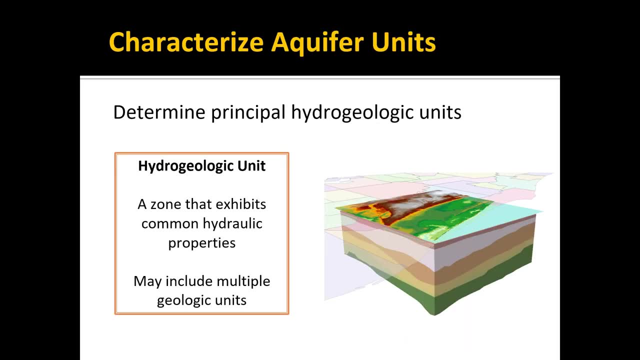 made as simple as possible, but not simpler. so that's just a another fun way of saying the thing, same thing that said at the top there. one of the fundamental parts of building a conceptual model is to characterize the, the aquifer units, the, the layering stratigraphy of your system, and to do 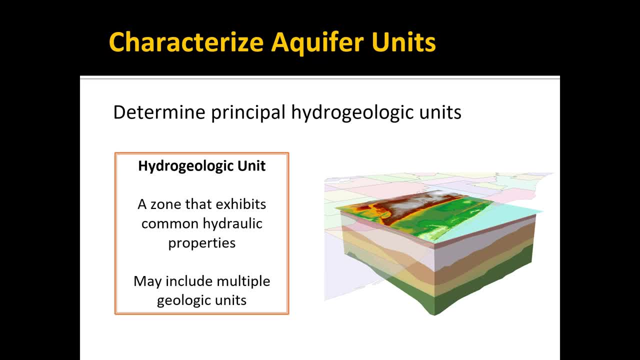 that we we call- we use this term- hydrogeologic unit, or it's often referred to as an HGU. you'll see that in a lot of the modeling literature, hydrogeological unit is is a unit as a zone that exhibits common hydraulic properties and it could. 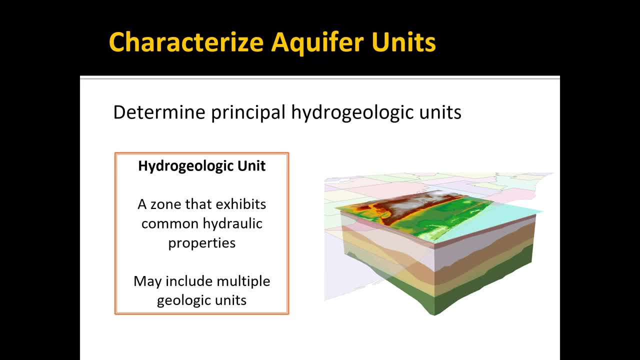 include multiple geologic units. it's defined on the basis of hydrogeology more than anything, and- and that that's one of the first things you have to do- this site shown on the right is a model stratigraphy model. I helped build for the south, the st. 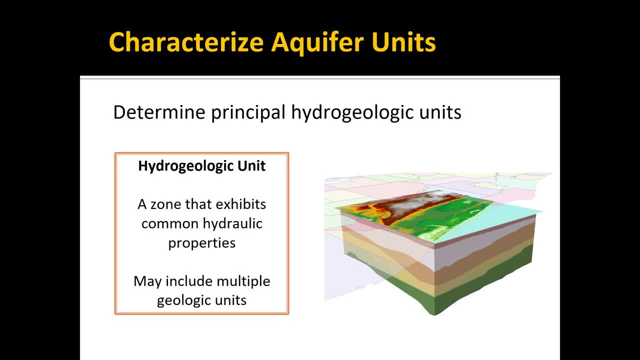 john's river water management district in Florida and they had a lot of well-logged data that they acquired over many years and were able to put that into this three-dimensional system that I helped develop that works inside ArcGIS, called our hydro groundwater and we built this model and here are some other examples. this is a 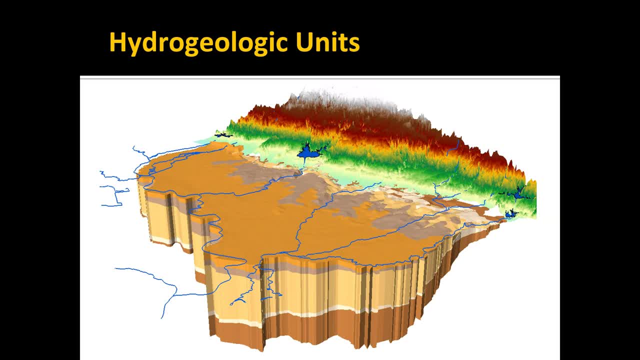 model in the Sacramento region of California, as part of the Central Valley, and back trying to remember the exact timeframe: maybe early 2000s, 2000 to 2005-2008, somewhere in there, I recall correctly, I worked with a local company, Aquavale, to build a computer. 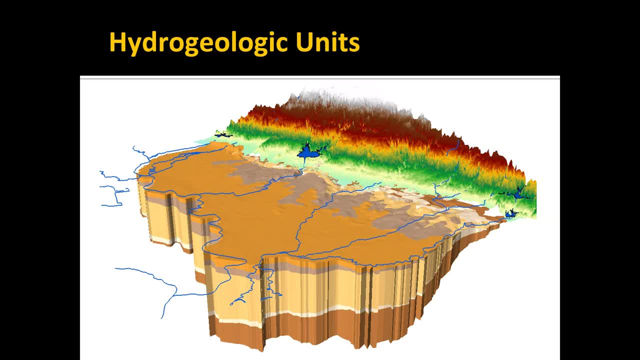 model with, with my colleague Michelle Smilowitz, to build them, model for the Sacramento region. and so the mountains you see there, the Sevier Nevada mountains, we have the Folsom River, Sacramento River, a bunch of the rivers in the region, and then again we use this arch hydro groundwater that 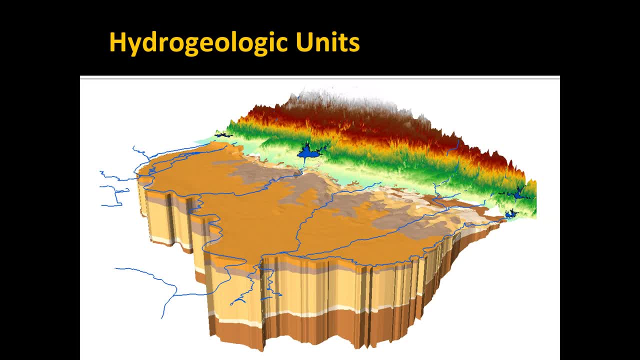 works in conjunction with with GMS and mod flow to build a model of the hydrostatigraphy and and so- and I think I reference this in one of our earlier discussions, but this, this top layer, is a very low permeability clay unit, and then we have a number of lower layers, that again, each of which includes smaller 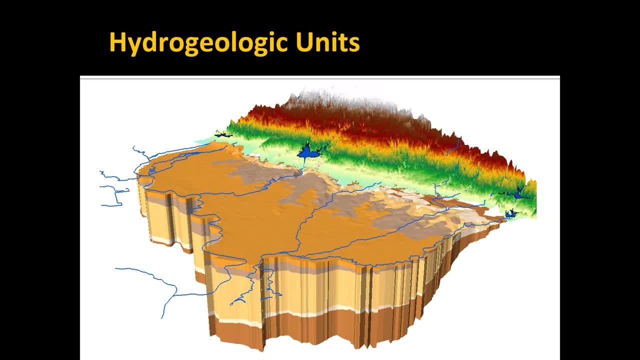 subunits, but these are classified based on overall permeability relative to the other units. and there was an earlier model in this region where the- the conceptual model they used- had this top clay layer going all the way over to the Sierra Nevada mountains over here. but as a matter of fact, there's this, these, these zones here. 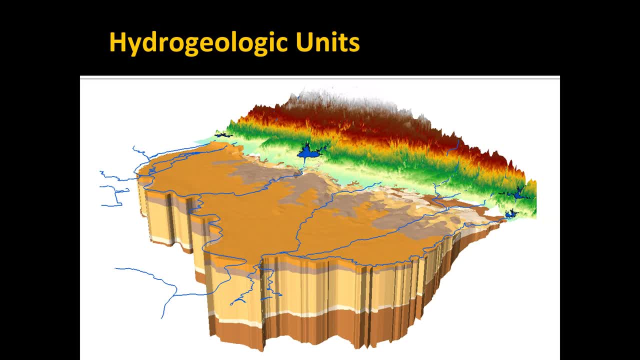 next to the mountains that that surface are a much higher permeability, and so a lot of the recharge in the region comes into these zones and percolates down the region to the lower layers, and so one of the objectives of building this model was to 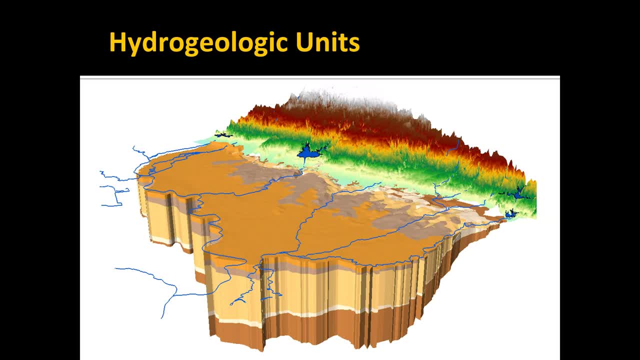 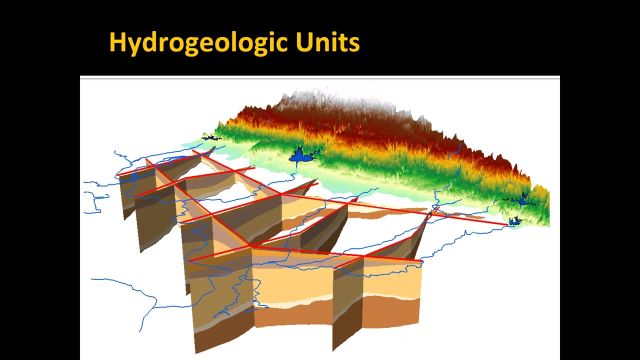 properly include that connection of those lower units with with the ground surface to better simulate that recharge. and so, again, that's part of building your conceptual model- is making sure you have those features represented the way you want. and this is just a series of cross sections that are cut through the 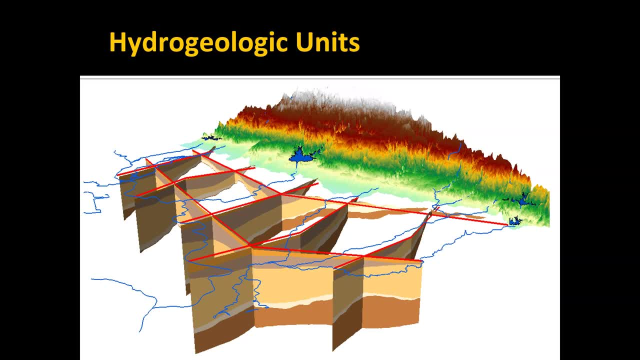 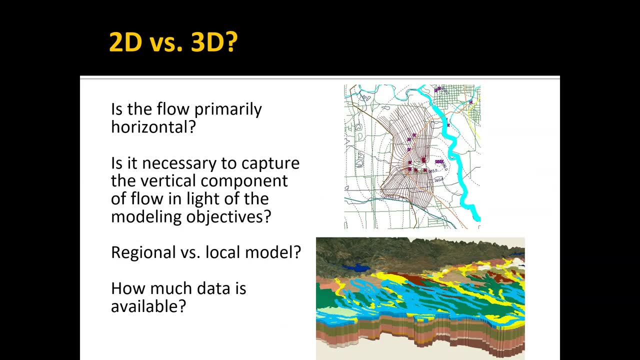 same hydrostatigraphy, but each of these layers were eventually included in our numerical model. another question you have to ask. oh, by the way, the the this figure here on the bottom, this is the three-dimensional numerical model that we eventually constructed using mod flow of this site, and this particular one had these blue lines. these are braided. 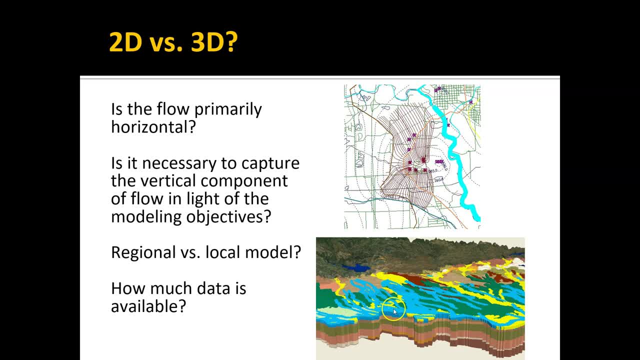 channels that are that were part of that upper unit. we took that upper unit and made it more detailed- and, incidentally, we built a model this way and then, based on feedback, we and and our model results, we decided that we weren't really gaining anything from having these stream channels and things inside that top. 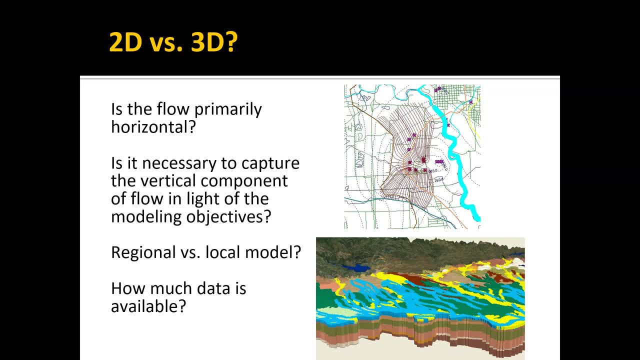 layer and so we took a lot of them out. so we actually added complexity and then removed the complexity because it wasn't making our model any better. so we went back to a simpler model. but again, that's part of it. Thank you, You can see the layering there of those hydrogeologic units from the previous images that we're 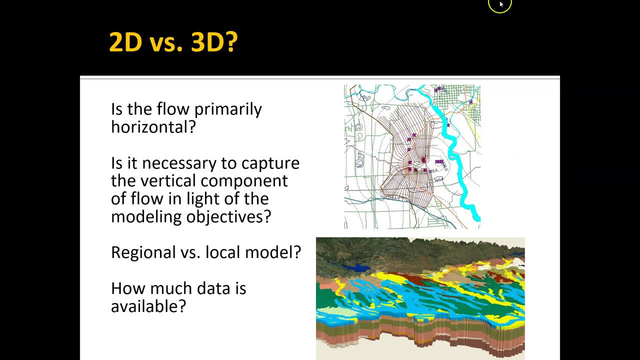 looking at now. sometimes we ask 2D versus 3D. well, in some cases we can get by with just a single layer model, just kind of a homogeneous layer. you don't have alternating layers of different hydraulic conductivity and we often refer to that as a two-dimensional model, because 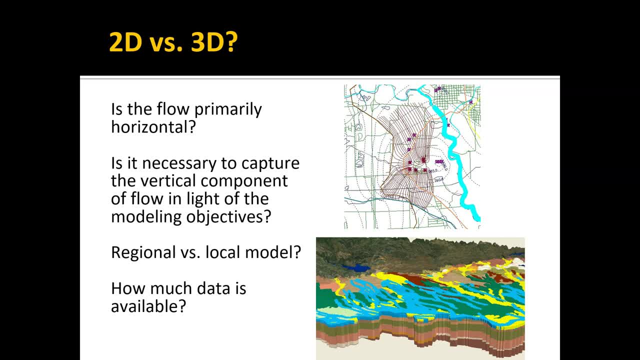 there's only one layer In the vertical direction. and how do you decide? well, if the flow is primarily horizontal and there's not that much differentiation in hydraulic conductivity vertically, or you don't really have a means of calibrating, you don't have water level observations at multiple depths. it's a lot of times. I would recommend going. 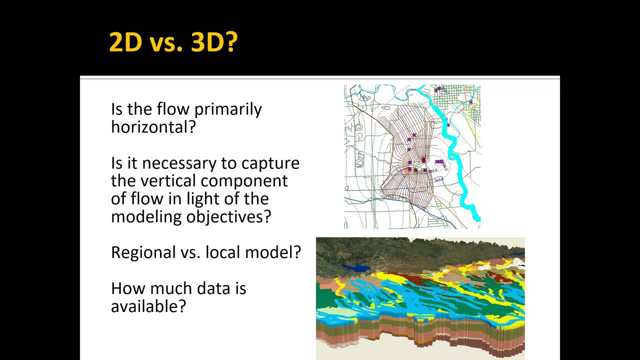 with a 2D model. It keeps things a lot simpler and you know is it. is it a regional model or local scale model? do you have enough data to support building something like shown on the bottom, or can you get by with just a simpler model as shown on the top? 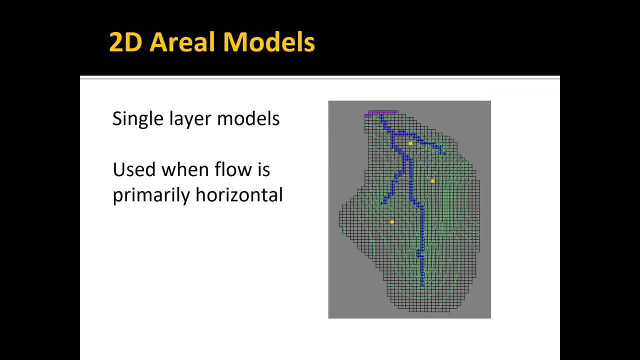 So that's one of the first things you need to decide as well. and again, this is an example of a two dimensional- I call it. we sometimes are called aerial models, because you're looking down on it in plan view, and so it's a single layer model where the flow is primarily 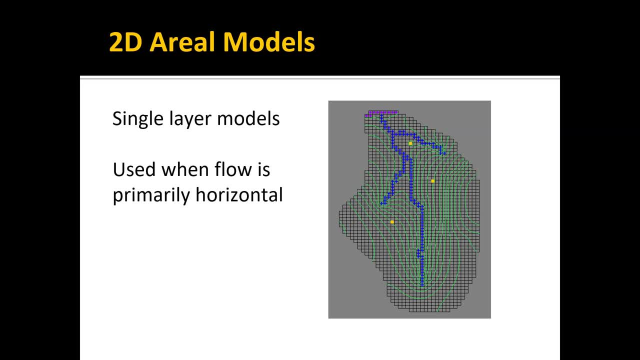 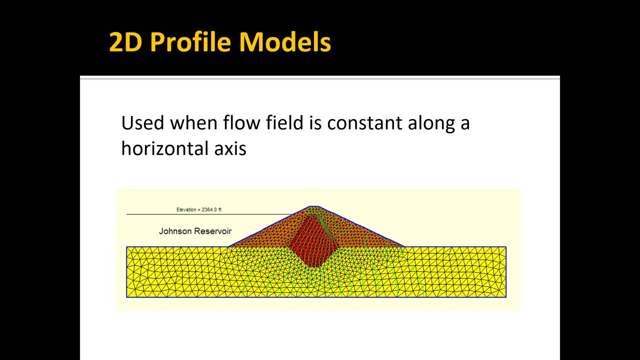 horizontal and we're going to be building a number of models or we're going to be doing several exercises involving this, the same model shown here. another form of a two-dimensional model is a profile model, and this is where you simulate flow along a vertical cross-section, and these are typically 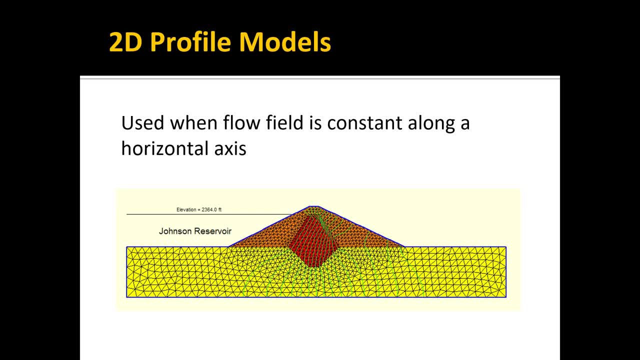 used when you're simulating the flow or seepage through a dam or a levee, and while this is an important part of designing dams and levees, the focus of this class is more on regional groundwater modeling, and so we're not going to be covering that. those of you who are 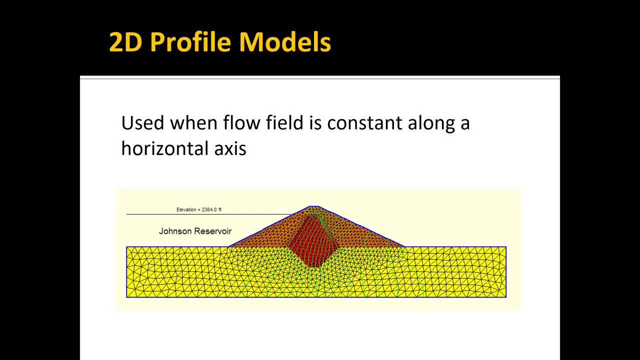 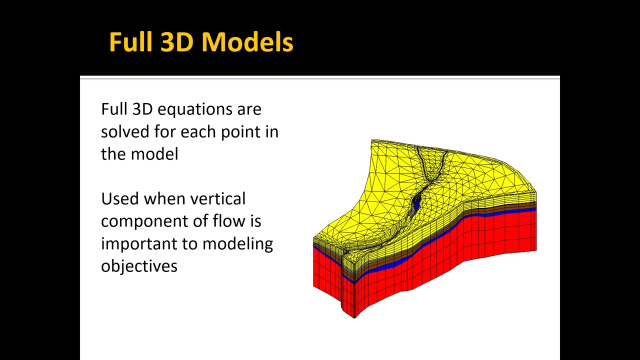 you students at Brigham Young University. in our department there's another course, CE 544- seepage analysis and seepage and slope stability analysis, where this cross-section models are featured quite heavily. and then of course you know you can have full 3d models. we've seen examples of that already now. another 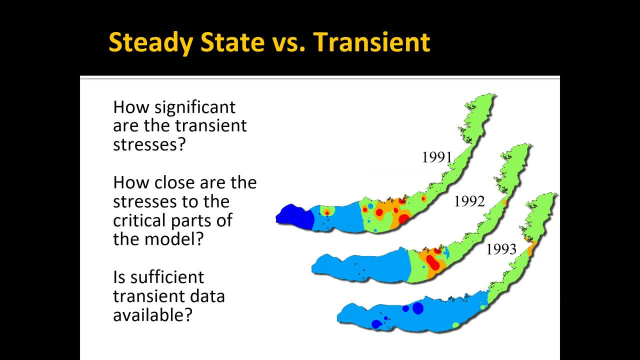 question you need to ask is: how do you simulate flow along a vertical cross-section needsa? that's what you all may be asking yourself. you need to ask is: are we going to do a steady state or transient model? steady state means you just pick some. 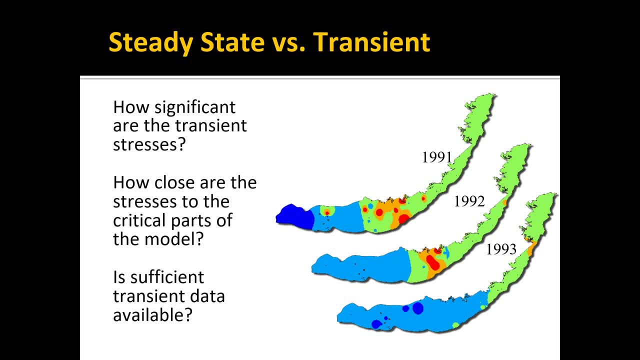 average conditions, and by conditions i mean recharge and pumping rates, maybe discharge to streams, and you kind of simulate a long-term average condition, whereas with a transient model any part of your sources and sinks can change. So things like hydraulic conductivity and the stratigraphy, those typically don't change. 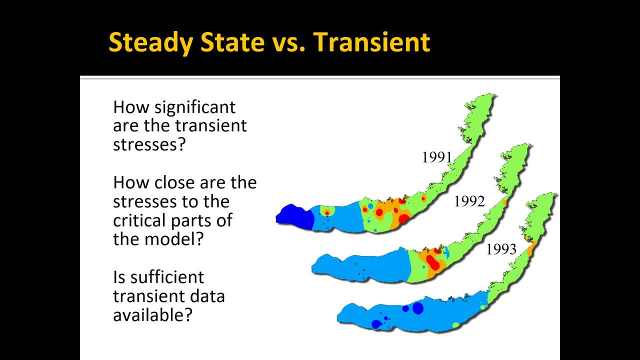 But how much water you're pumping from wells. some wells are turned off and on. That can vary over time. Certainly, your recharge can vary over time, And those things can all be entered into a transient model. Now it's very important to emphasize here that there is no such thing in nature as a truly steady-state groundwater system. 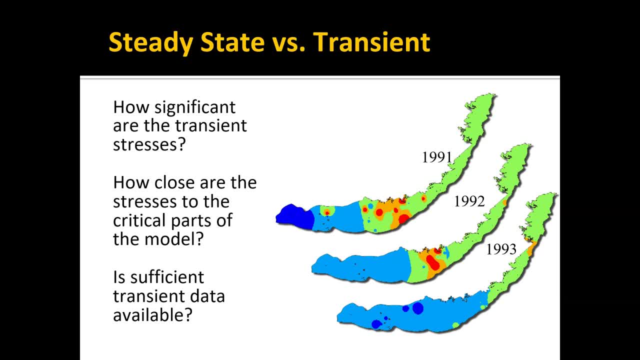 They're all dynamic to some extent, And so you know why would you ever do a steady-state model? Well, again, it comes back to your modeling objectives and how much data you have. Steady-state models are a lot easier to calibrate. 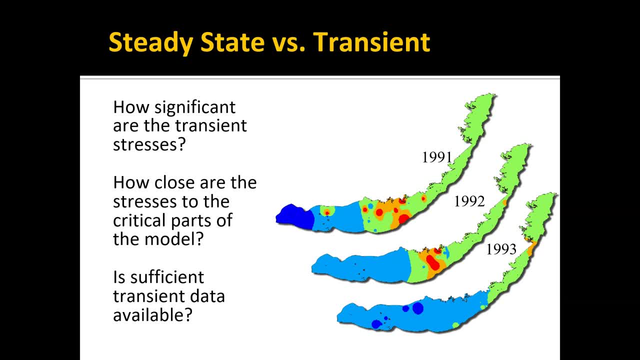 Well easier in the sense that the models run rapidly and you can calibrate the model fairly quickly. A lot of times you'll have a model that will run in maybe 10,, 20, 30 seconds in steady-state, But if you make it transient it could take well 15, 30 minutes, maybe an hour to run. 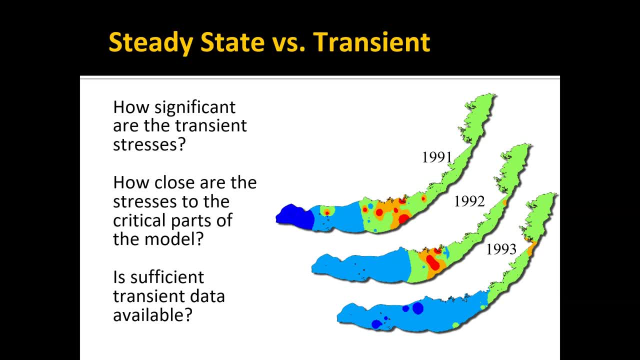 And so that obviously is going to take longer to calibrate. And again it depends on your objectives. If you have transient data, transient observations that you can calibrate to, then you typically want to do that. I would say most groundwater modeling projects you end up with a transient model. 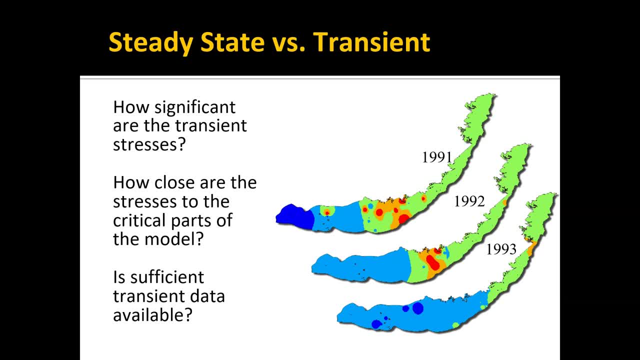 Sometimes we build a steady-state model as a stepping stone on the way to a transient model. We calibrate to steady-state conditions and then take those results and refine it further as we calibrate to transient conditions, And then we almost always- And when we can end up with a predictive model, that's almost always a transient model. 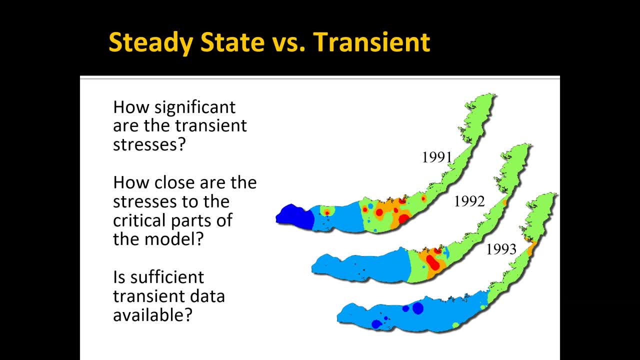 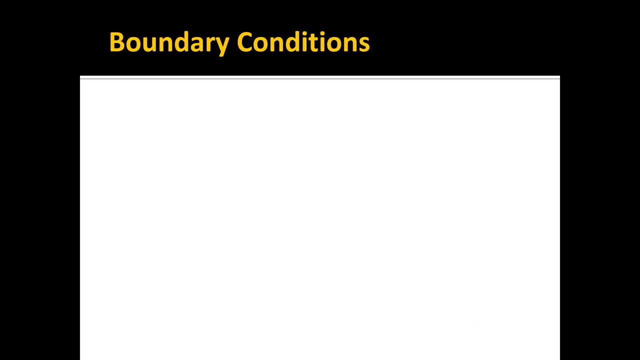 So you're looking at changing conditions going forward. Okay, another thing that you have to decide as part of your conceptual model- one of the most important parts- is your boundary conditions. How far do you extend your model laterally and vertically, and what do you use for your boundaries? 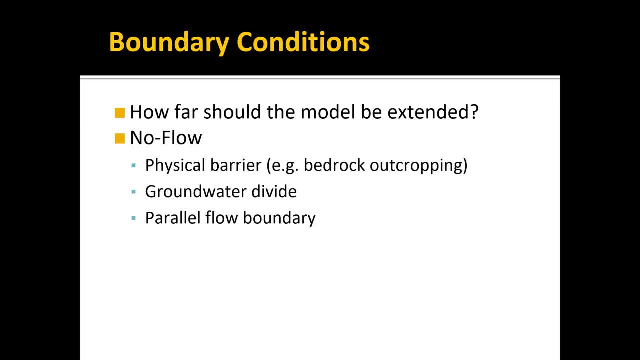 That's a really important question, and what are some typical boundary conditions? Well, one type of boundary condition is what we call a no-flow boundary condition, and these are pretty intuitive. This would be, for example, a physical barrier. Maybe at the edge of your aquifer you have a bedrock outcropping. 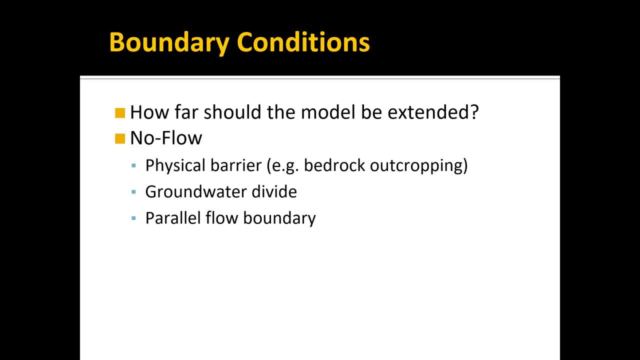 We typically get these when we're simulating flow in alluvial systems in a valley next to a mountain, A mountain range or something, but there are some others as well. A groundwater divide is where you have a location in your aquifer where on one side of the divide the groundwater flows to the north. 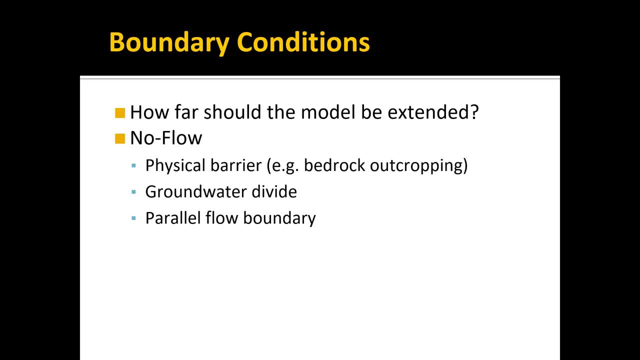 On the other divide it flows to the south. It would be like a ridge in your water table and you can treat that as a no-flow boundary, Or a parallel flow. boundary is if the water's flowing in a certain direction. if you slice a line in that direction, you can make that a no-flow boundary. 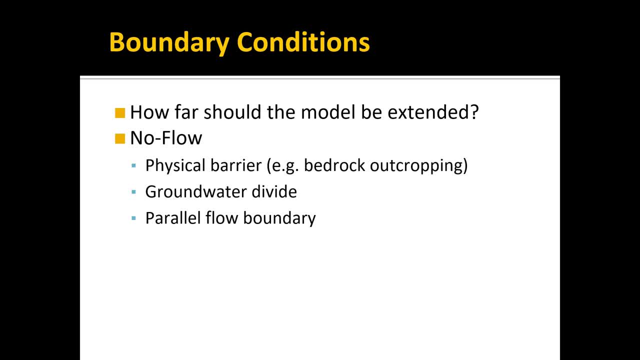 The physical barrier is the best kind of no-flow boundary, but sometimes you have to use the others as well, and we're going to talk more about those a little bit later in this semester. Another really common, important kind of boundary condition is a head dependent, or is a head-based boundary condition. 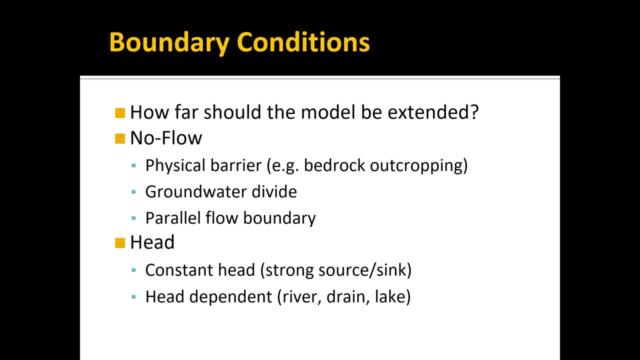 Sometimes we call this a constant head or a fixed head boundary condition. This is where you have a really strong source or sink, And when I say that I mean a lake or a river that intersects with our aquifer, with our water table, and provides a fixed water level at that part of the aquifer where it's connected to the lake or river. 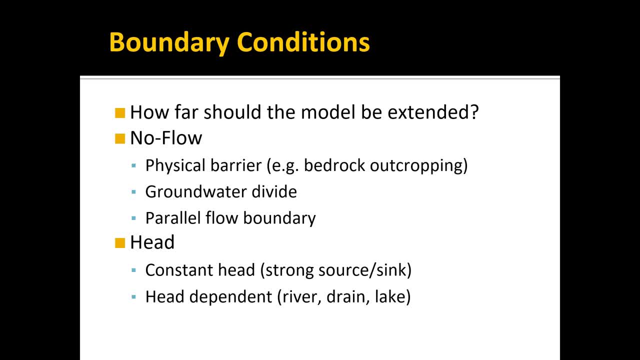 And those are constant head-bounded conditions. And another Variant of that is a head-dependent boundary condition and that could be a river drain or a lake. that doesn't absolutely fix the head in the aquifer but it strongly influences it. 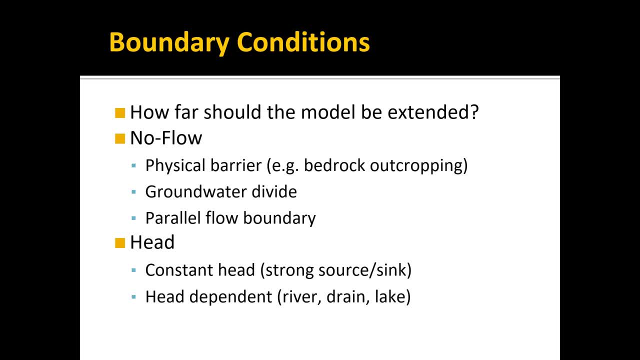 And we're going to look at a number of those as we go on this semester. So when you're developing your conceptual model, sometimes you extend your boundary out to a river Or to a lake or some other feature where you have constant head or head-dependent conditions. 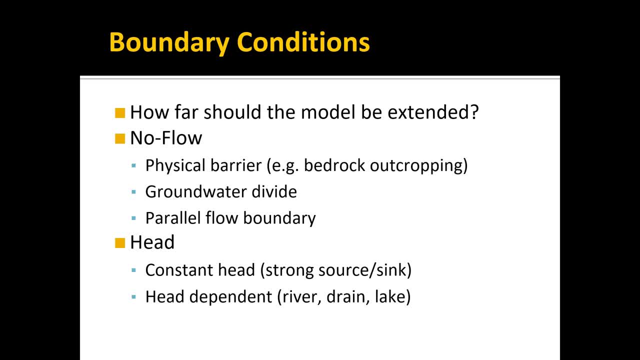 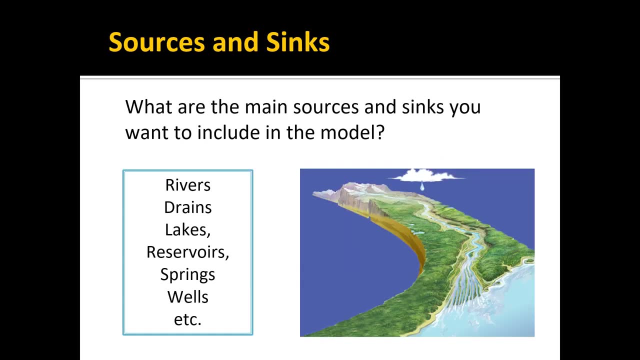 In other cases you extend it out to some kind of physical barrier, But typically one of these five types listed here is what corresponds to each of the boundaries on your groundwater model. I've used the term source and sink a lot. I just want to make sure it's clear what we mean by that. 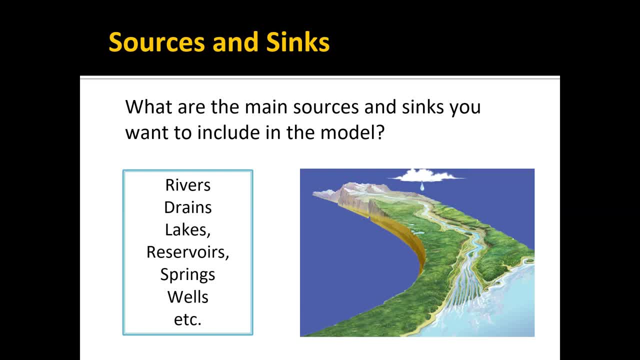 Source or a sink is a feature that can either add water to the aquifer or drain water from the aquifer, And so, again, the most obvious examples of that would be a river, a lake, a reservoir, A river- you've probably heard the term- a gaining river and a losing river. 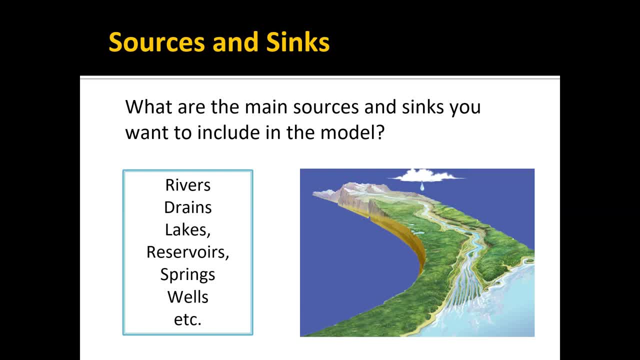 A gaining river means that as the river moves along, it gains water, And that is typically from seepage to the river, from the aquifer, And so, from the aquifer's viewpoint, water is that would be a sink, because water is leaving the aquifer into the river. 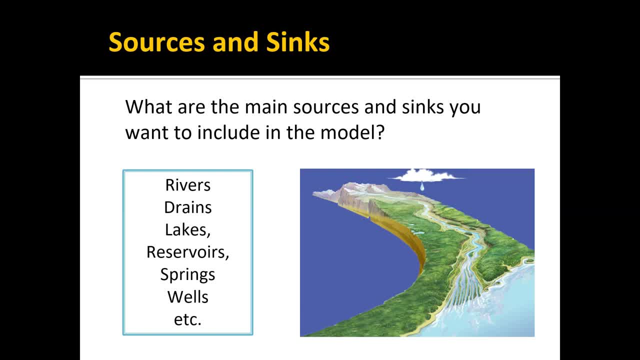 And then sometimes we have losing rivers, where water is lost from the river to the aquifer And we would call that a source, because it's a source of water to the aquifer. So this naming convention really depends on on the perspective of: are you looking at it from the viewpoint of the aquifer or from the external water body? 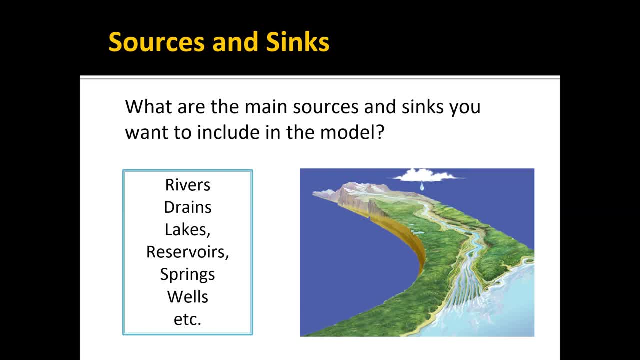 And again, you can have drainage at the bottom of a lake or reservoir or you can have an aquifer that basically feeds the flow of water into a lake or reservoir. A spring is always a sink. It's basically where you have The water table is high. 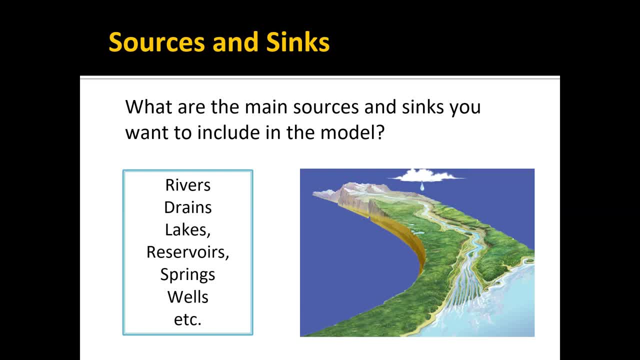 Maybe it's even under artesian conditions and the water is flowing freely to the ground surface Well, it can be a source or a sink, but the vast majority of wells are extraction wells, and so they're sinks. Another one that I have listed here is a drain. 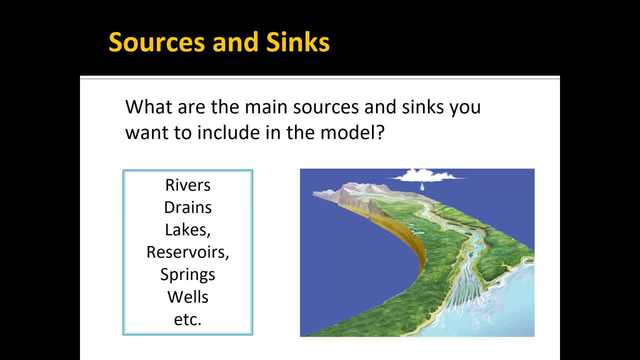 A drain would be. It's always a sink. It's a feature where if the water table is high enough, it discharges, But if the water table is low it doesn't discharge. And you can think of, Suppose you had a. 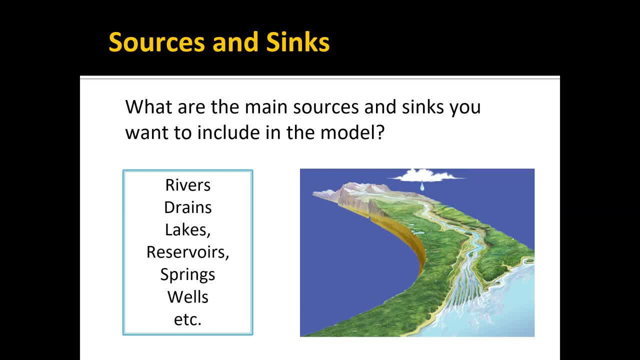 You know a mountain aquifer and you have a ravine. At periods where the water table is high maybe water discharges into that ravine and drains water from the aquifer. But when it's dry and the water table is low, maybe it goes. 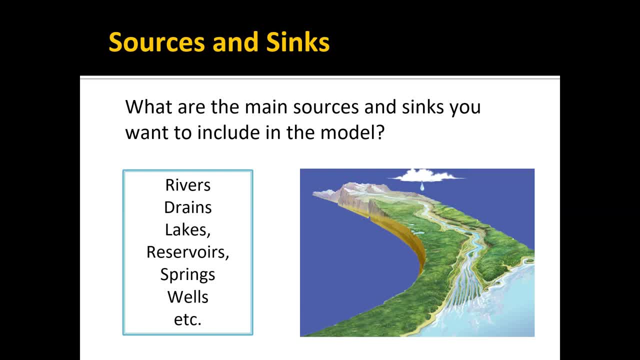 During a dry period maybe that ravine goes dry and water doesn't flow. So ephemeral streams is another way to put that. It could also correspond to seeps or wet periods near a lake. If the water level is high enough, it seeps out around the edge of the lake into the lake. 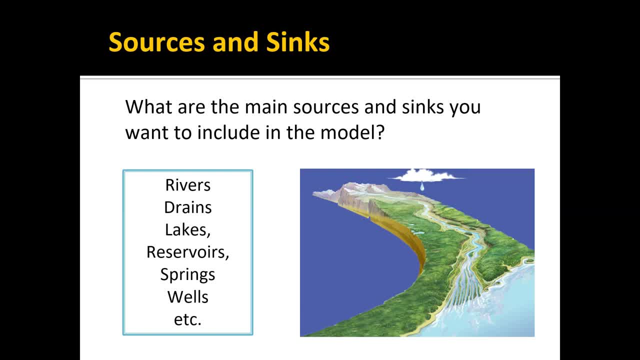 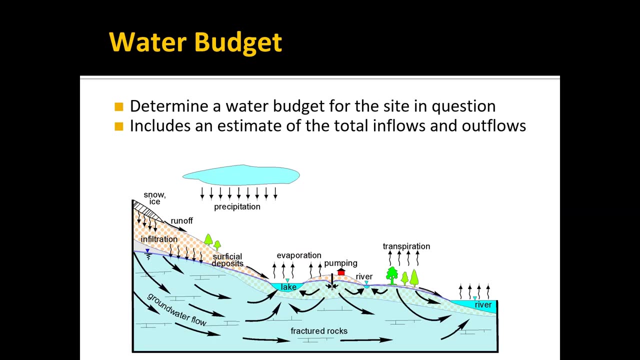 A number of different things can be classified as a drain, And those all need to be identified, And some of those are small and insignificant, But others are large and significant enough that they need to be included in the model. Now, finally, once you consider all these different things, 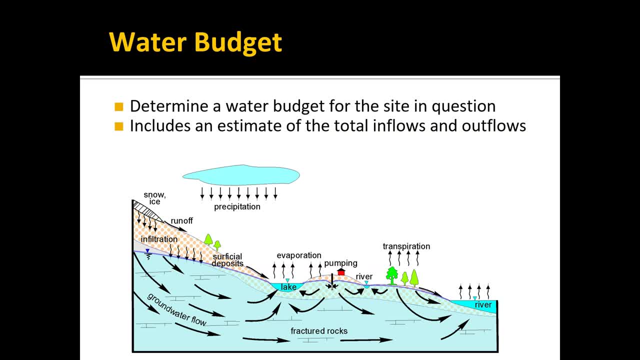 your boundary conditions, your layering, the sources and sinks that you're going to include. one of the most fundamental parts of building a conception model is to analyze your flow budget, So this means that we look at basically all of the ways that water could go into the aquifer. 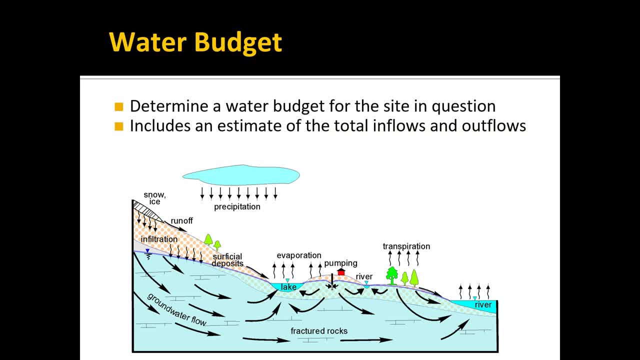 and all of the ways that it could go out of the aquifer And we come up with. You know, sometimes it ends up being just a representation, a graphical representation so that we get an understanding, And other times people will actually try to put numbers on that and estimate what the quantities are. 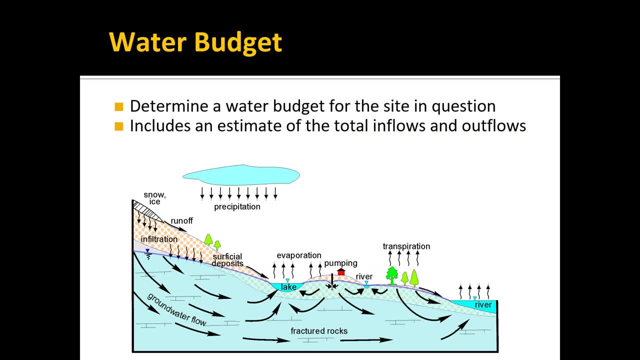 So here's an example: a cross-section through a site. We have precipitation, part of which can turn into infiltration. There's snow and ice which melts, And there's another source of infiltration: The groundwater flow. some of it discharges to a lake. 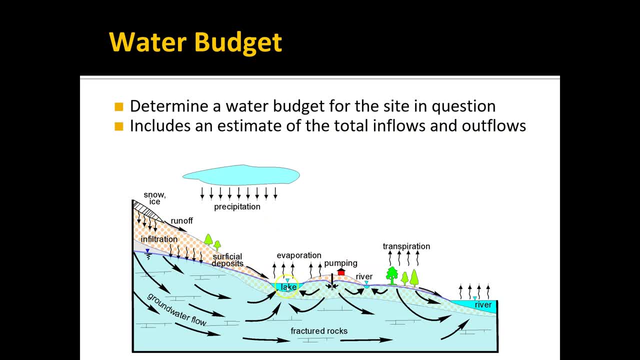 which then has some evaporation and drainage from the lake. presumably We have water that's lost to pumping And hopefully you can quantify that. Sometimes that's hard to do, but you do have to get an estimate of what the pumping rate is. 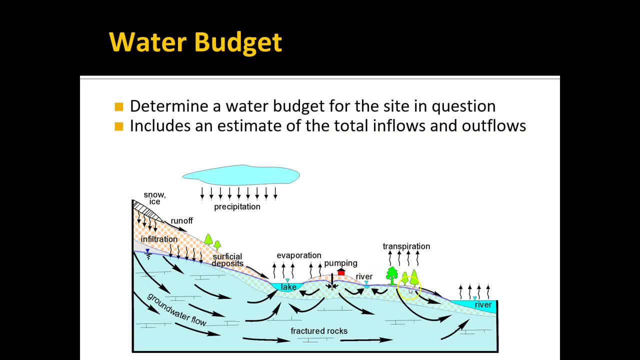 Some water is discharged to the stream, There's some transpiration to plants And discharge to multiple streams and flow through fractured rock. And again. developing a flow budget or a water budget has two purposes: both to characterize your assumed direction of flow with all of your external sources and sinks. 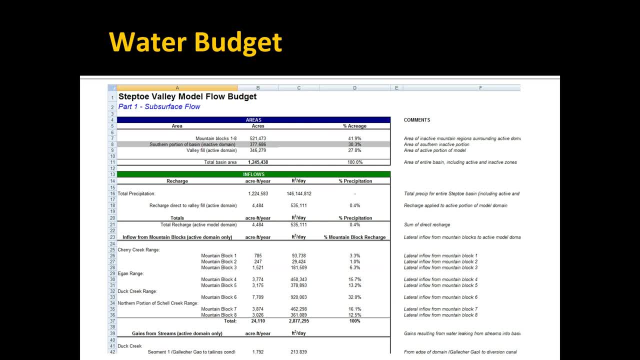 and sometimes an attempt to quantify that. So this is another modeling project I was involved with for a model in Steptoe Valley in Nevada And in this case, before we even built the numerical model, we developed a spreadsheet. We had it sketched out, of course, graphically and conceptually.